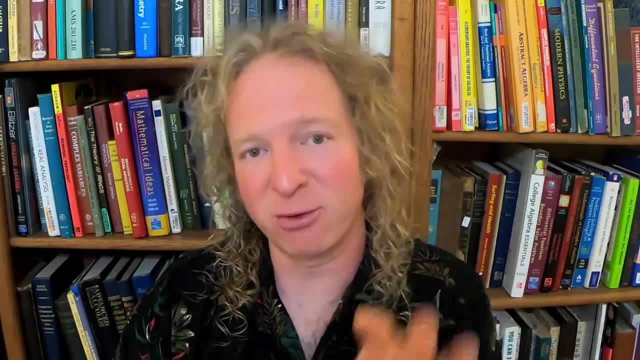 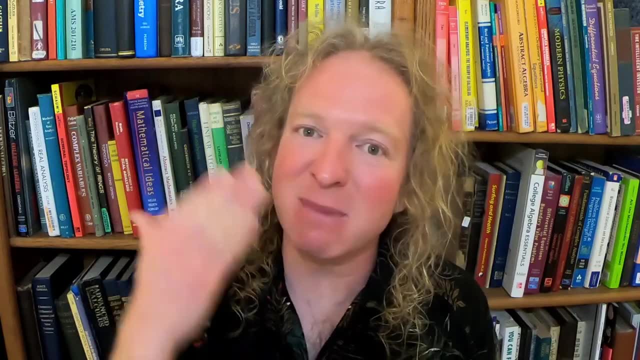 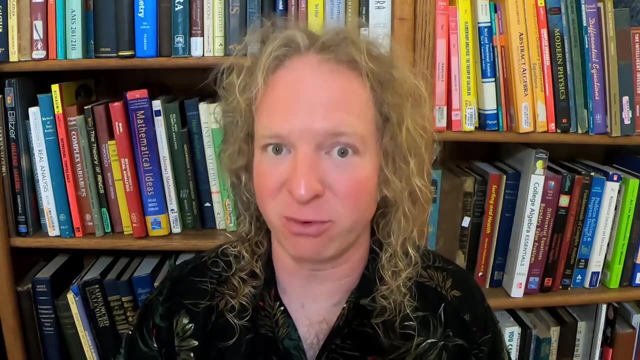 proof. But if you don't, the next best thing is to find a proof on the internet or in a book and then compare it to yours And then make sure your proof follows the same exact logical steps. So, once you know that your proof is correct, here's what you can do to get better at proof writing. You go through your proof. 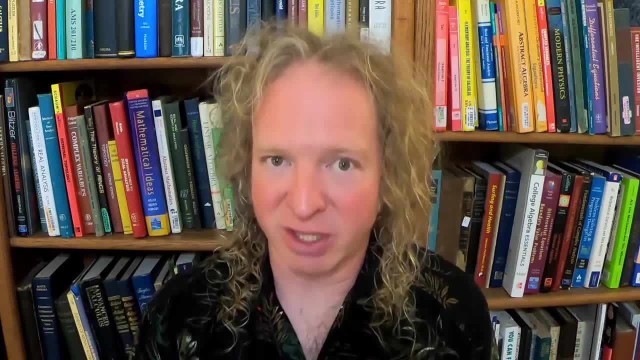 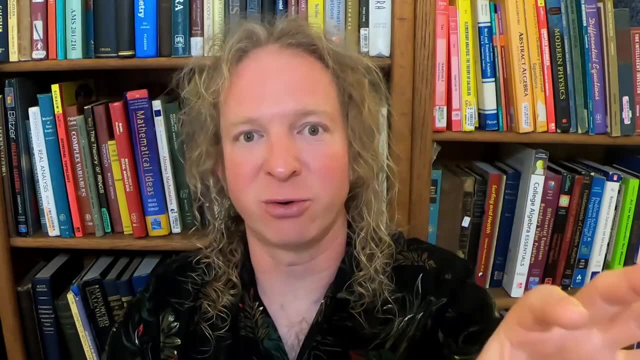 and you really think about every step. okay, You try to think about the structure of the proof. Look at your hypothesis, where you started your proof. You started with your hypothesis, your assumption, So like, if you're doing like an if-then proof, you know. 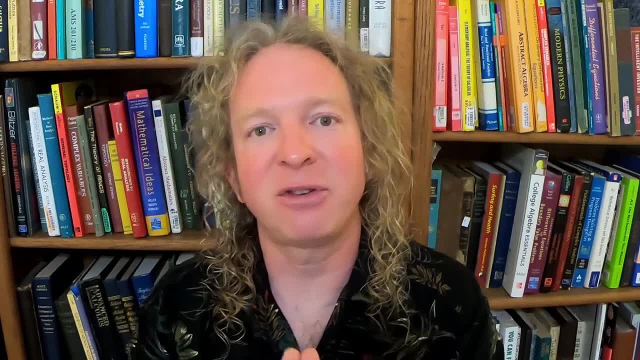 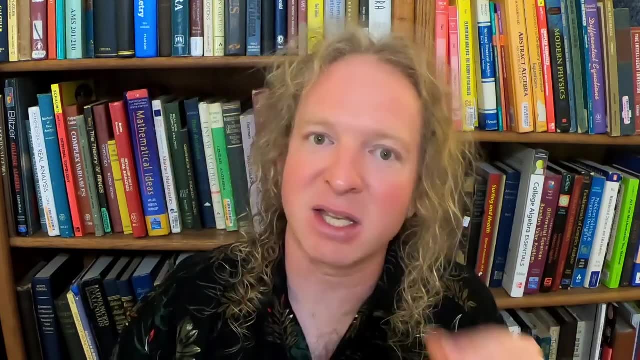 I don't know, And then think about what your next step was After you wrote down your hypothesis. what was your next step? You know, did you use the definition of your hypothesis A lot of times? that's the case. A lot of times you'll start a proof by saying: you know, I'll just make something. 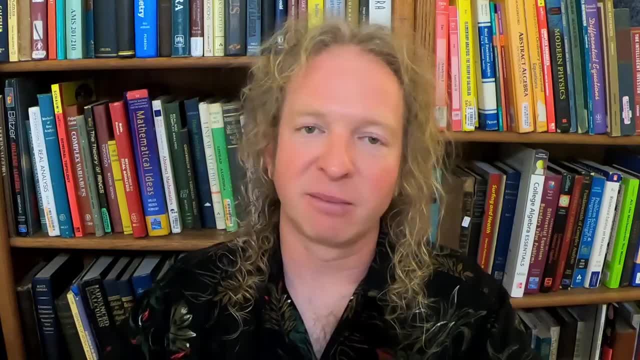 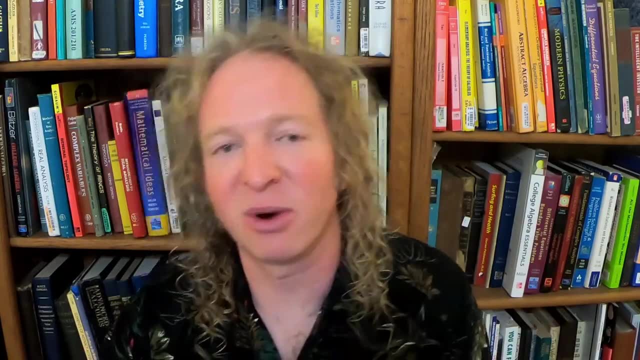 up. You know, suppose X is a BVD, whatever a BVD is, and making it up, So suppose X is a BVD, Then you write down what a BVD is right. So a lot of times it's all you do. Maybe you had to. 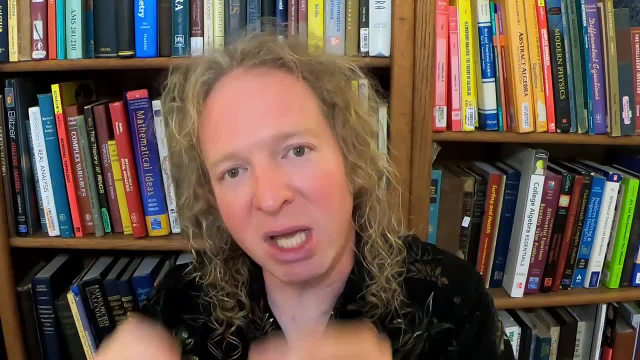 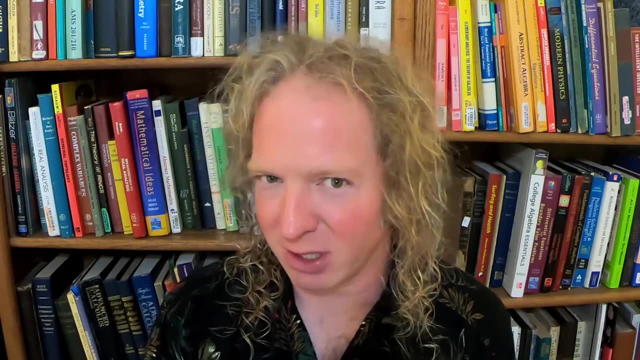 use the definition more than one. So just really really sit down and analyze your proofs And I find that if I don't tell myself to do this, I won't do it, And you might not be doing it either. Maybe you haven't, If you haven't. 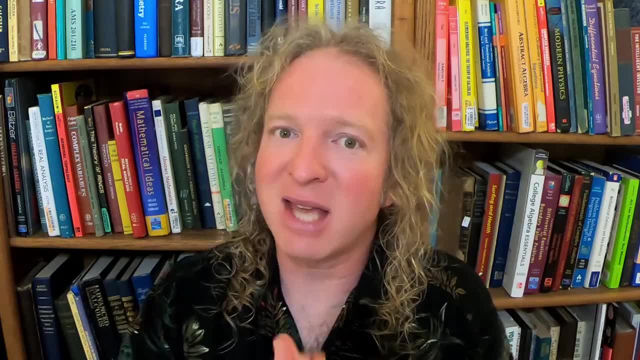 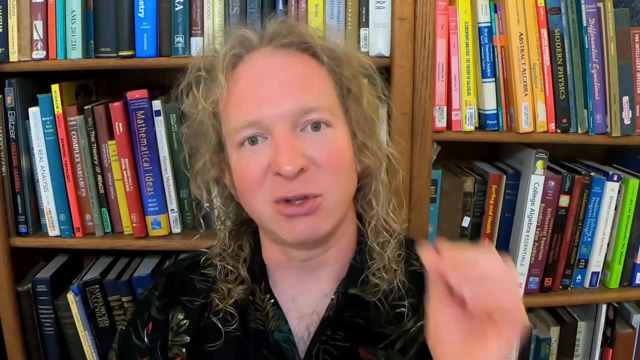 start doing it And I think the reason is it takes a lot of work to write a proof and figure out a proof. So once you figure it out and you know it's correct and you turn it in for a homework assignment or whatever and you get it back and it's correct, you put it away And again. 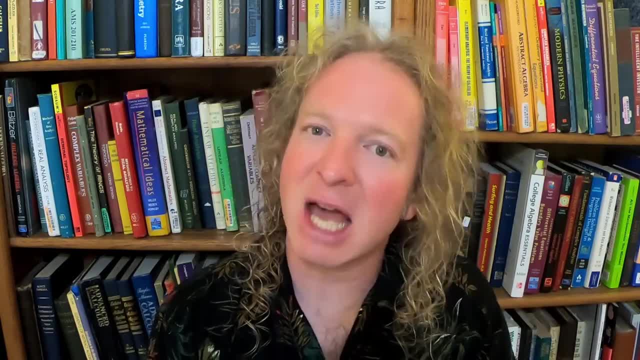 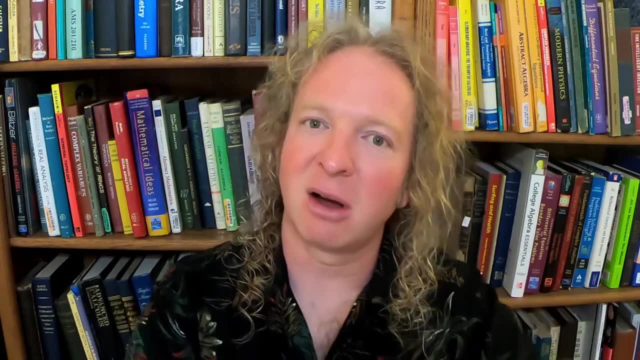 It goes in a folder and you never look at it again. right? That's not how it works. The best way to get really good at proof writing is to really reflect on your work and think about every single step. This is not my idea, right? 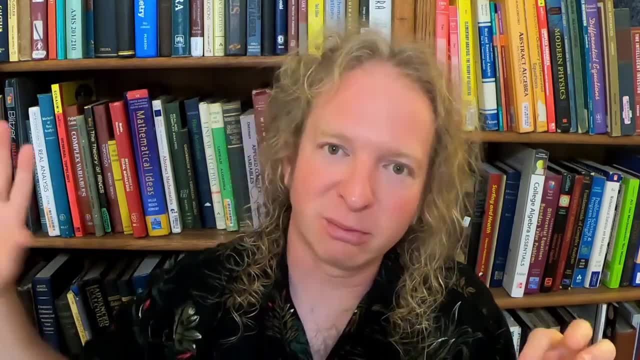 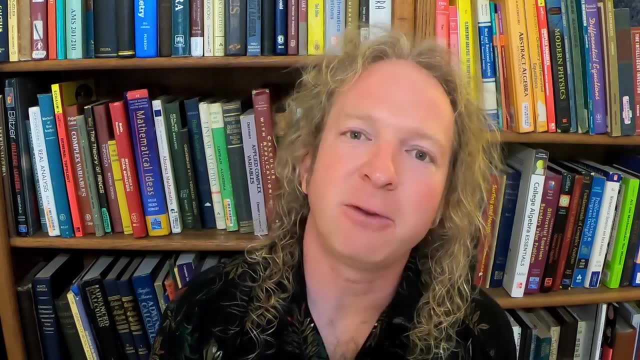 This is not my idea. I got this from a professor who passed away. He was semi-famous and I was fortunate to take his class. Same thing with induction proofs too. you know Like if you're doing an induction proof, always go back to the part. 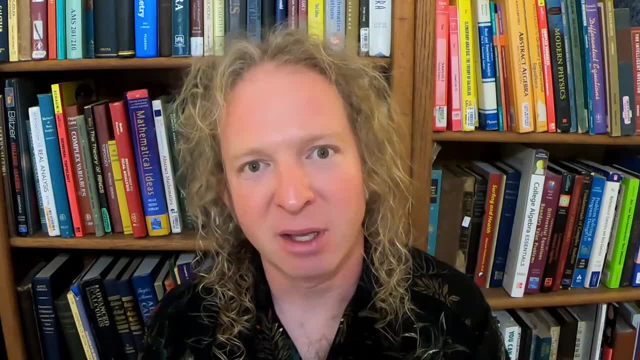 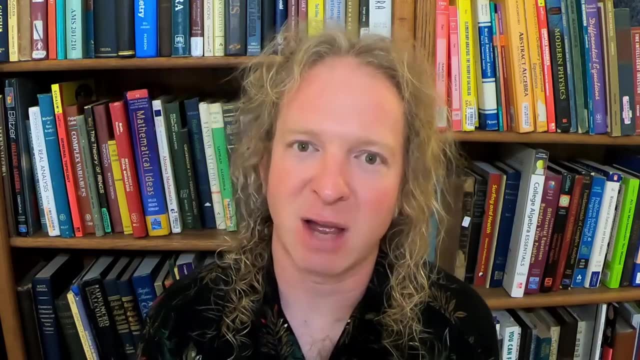 where you use the induction hypothesis and just analyze that part, And he would say, in that step of the proof, ask yourself what happens if you don't have the induction hypothesis. Why doesn't it work? Then think, okay, can I make it work without the hypothesis? 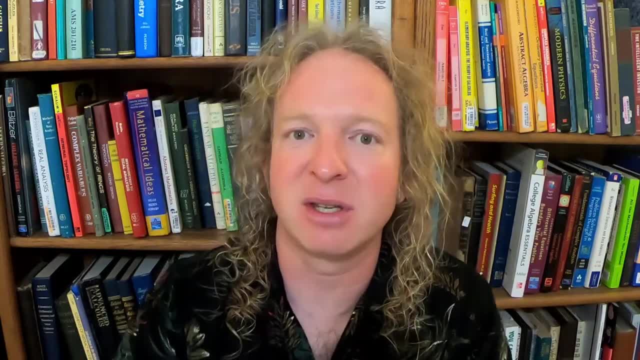 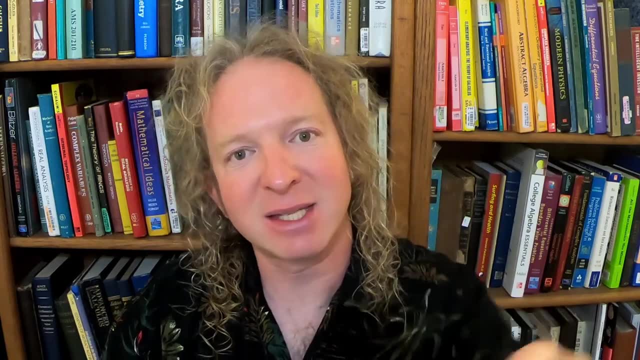 You won't be able to right. You won't Because you need the induction hypothesis, And he would always say that that was the beautiful thing about the induction proofs is that if you try to take away that step, it just falls apart. 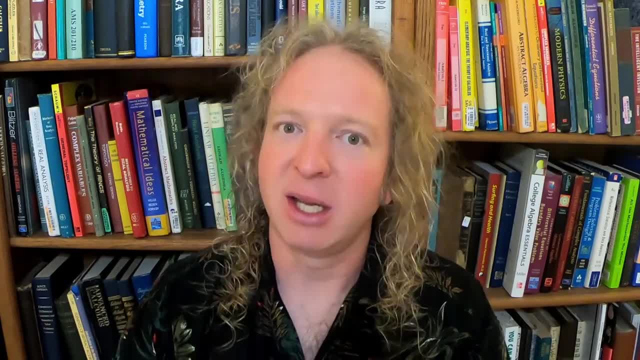 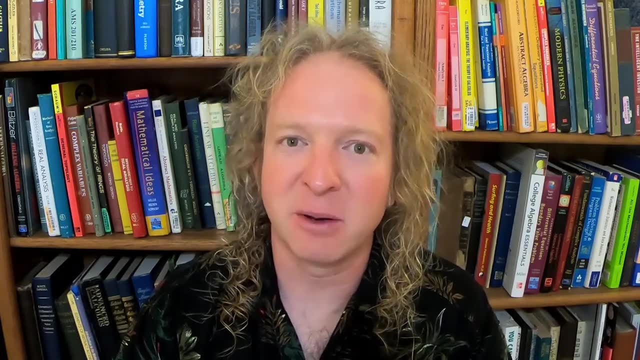 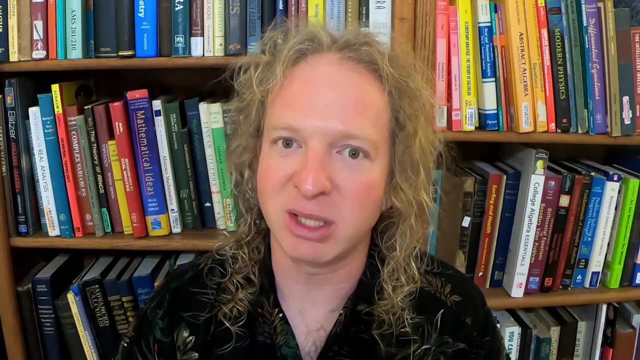 Analyze why it falls apart, right? Really, really, really good stuff. So I just wanted to make this short video and just talk about that, Because I think I remember his words. you know, Reflect on your proofs and just really, really, really deep. 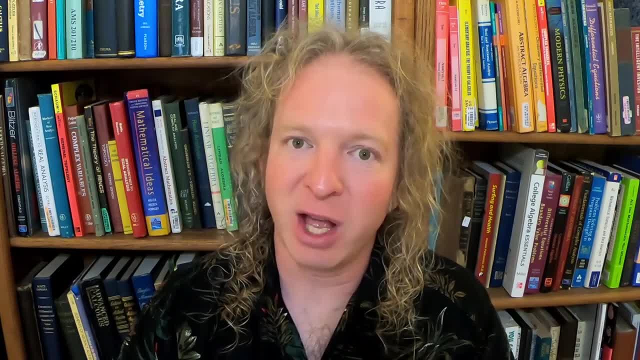 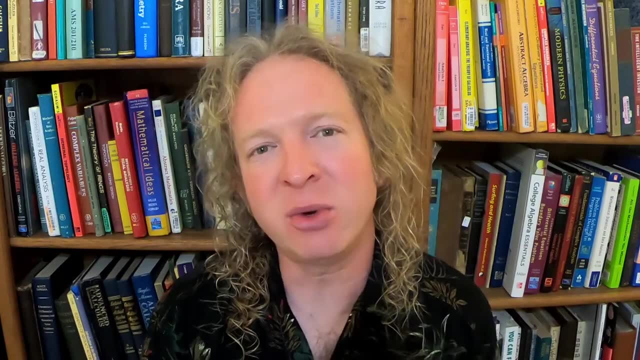 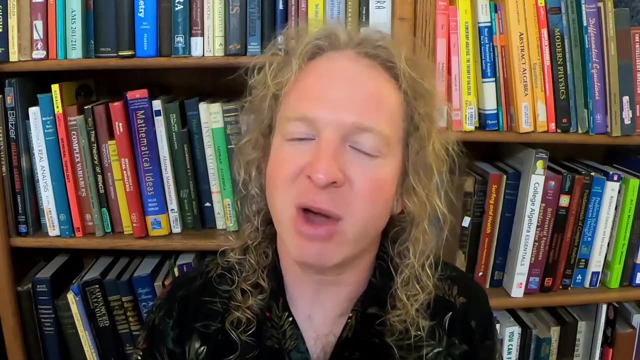 When you really start looking at proofs and the structure of proofs, you start to notice patterns and you start to notice similarities, And so by doing this reflection, you can employ those strategies into future proofs, For example whenever you have a finite set. 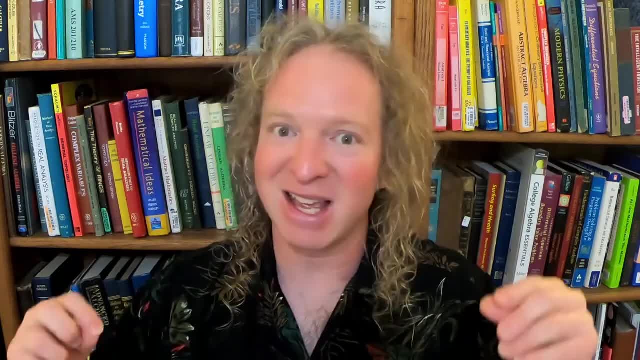 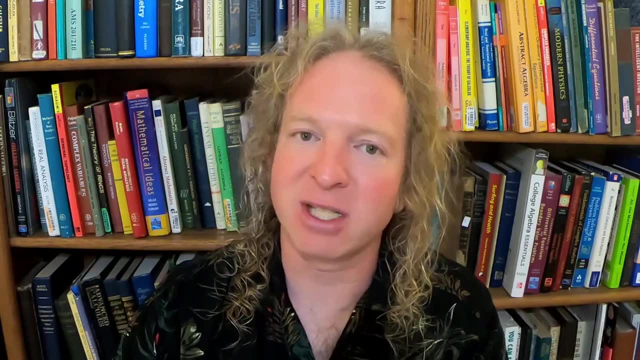 you can always take the maximum of that set. That is a reoccurring theme in mathematics, right? If you have a finite set, you can take the maximum of that set. For example, in real analysis, when you're trying to prove a convergent sequence is bounded. 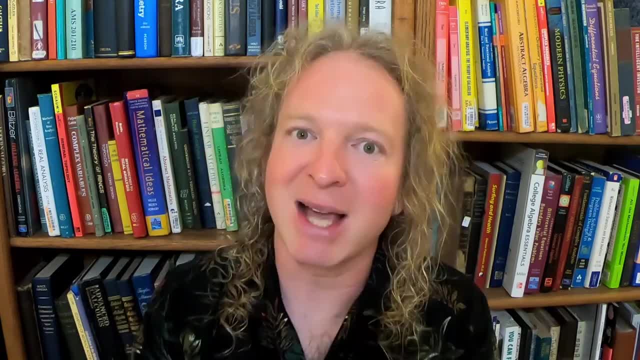 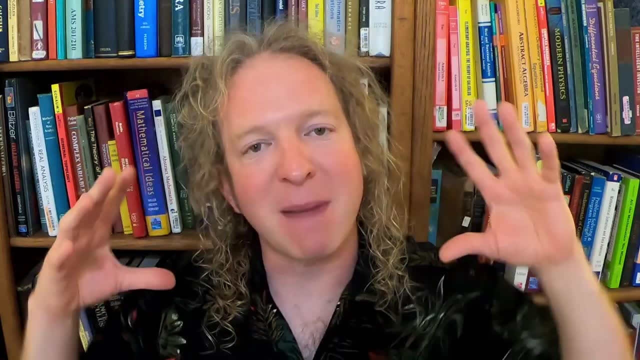 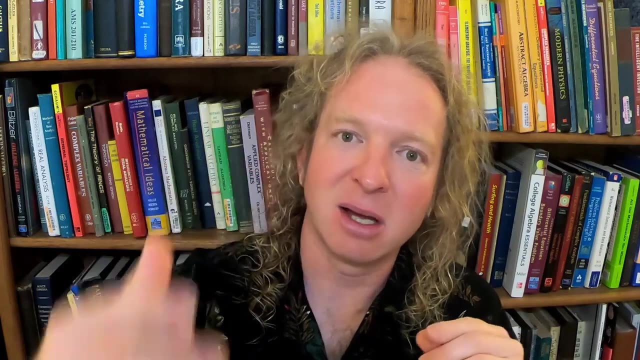 every convergent sequence is bounded. that proof right is bound. It relies on that right. There are several proofs in topology that also rely on that, on taking the maximum of a set. So little things like that, these reoccurring ideas. 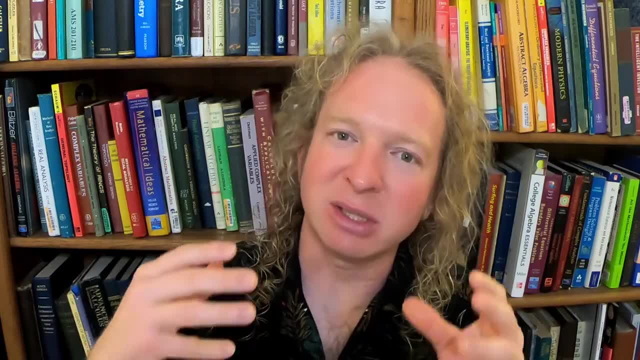 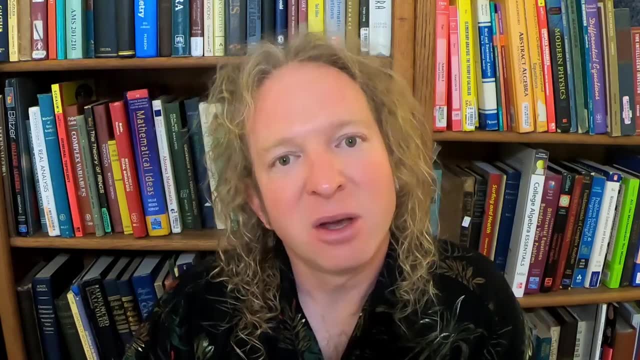 come up again and again. So really sit down and just go line by line and just reflect on the proof. Can it be written a different way? Sometimes you can prove it a different way. Can you prove it via contrapositive? What about a proof? 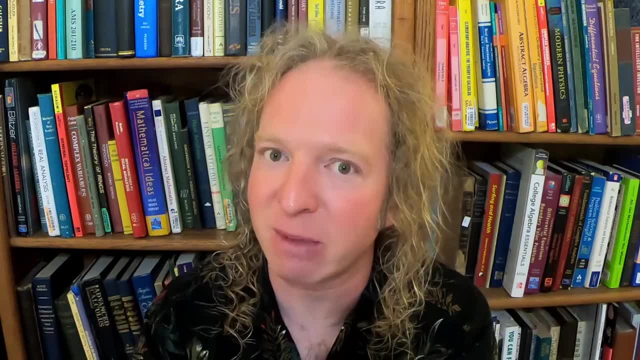 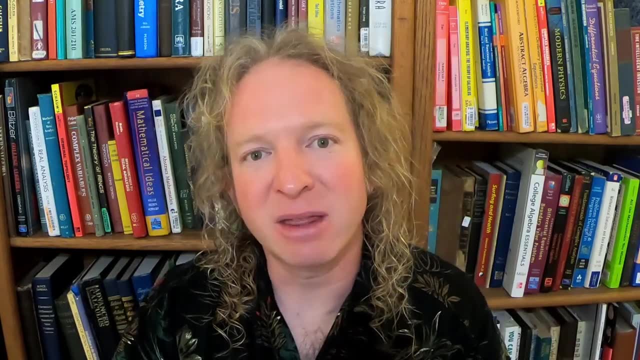 By contradiction, you know. Can you prove a stronger statement, right? Is there something stronger? Can you prove something even stronger than what you've just proven? And again, a lot of times, I think that we don't do that because we have time constraints, right?